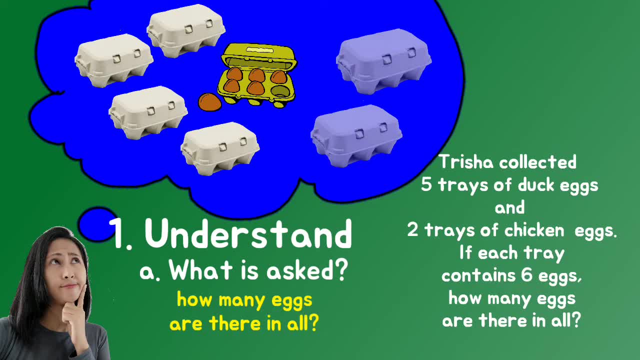 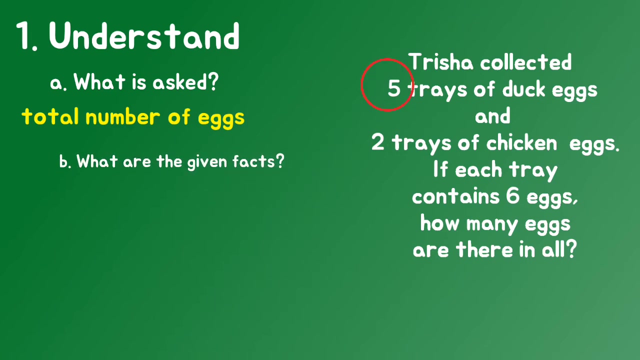 this, This, But if you can't construct a better phrase or a sentence, the idea will be like this: You can say this, This: What are the given facts? Remember, given facts are important numbers in the problem. given facts are important numbers in the problem. 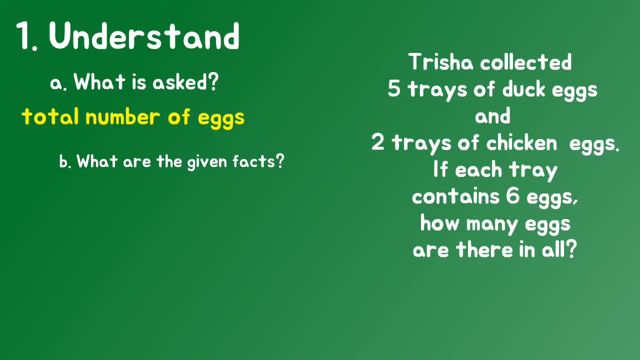 given facts are important numbers in the problem. These numbers are used to solve the problem. Given facts are 5 trays of duck eggs, 2 trays of chicken eggs and 6 eggs each tray. Then we have to make a plan What operation to be used. 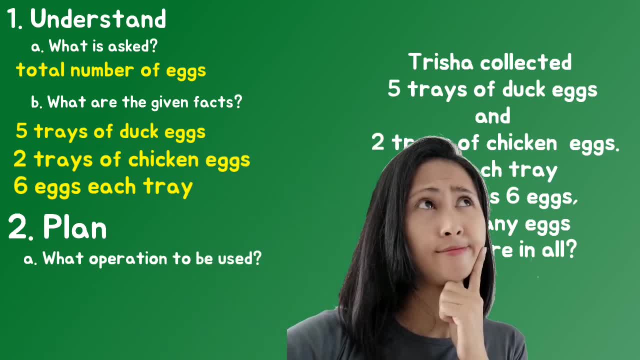 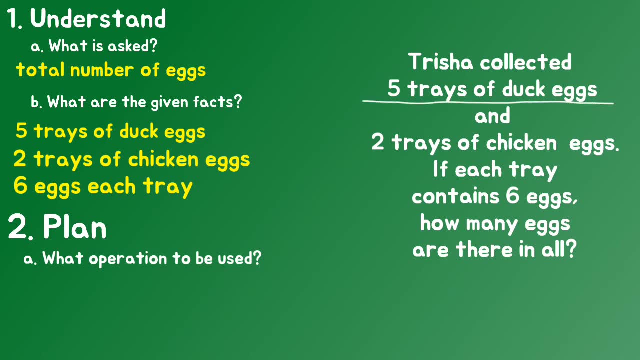 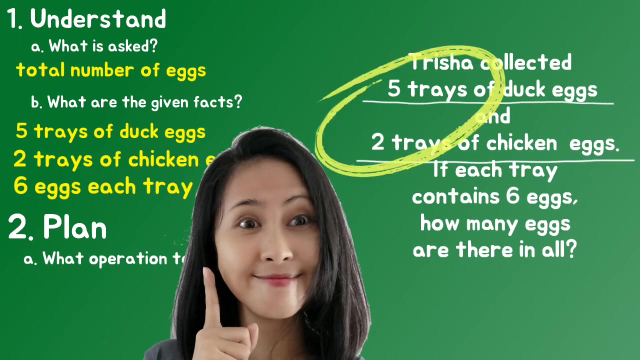 Which word suggests that we need to multiply, add or subtract In the problem? you can see that Tricia has collected 5 trays of duck eggs and 2 trays of chicken eggs. What is this information telling us? Oh, we need to know the total number of trays. 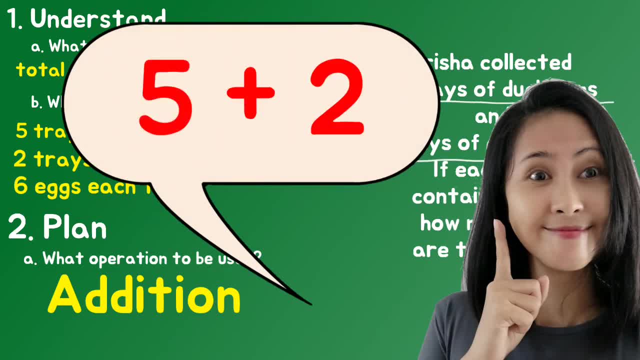 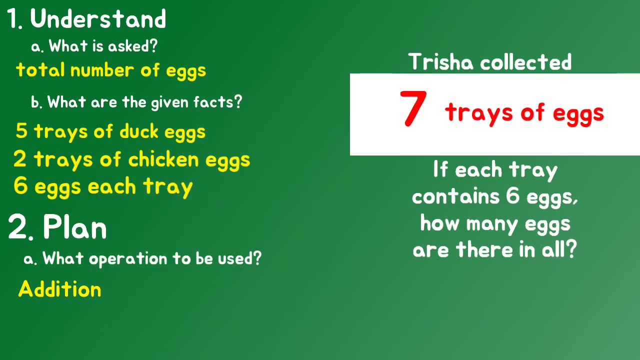 Aha, Addition 7 trays of eggs. Now it means Tricia collected 7 trays of eggs. If each tray contains 6 eggs, how many eggs are there in all? So how will we now get the total number of eggs? Let's search again. 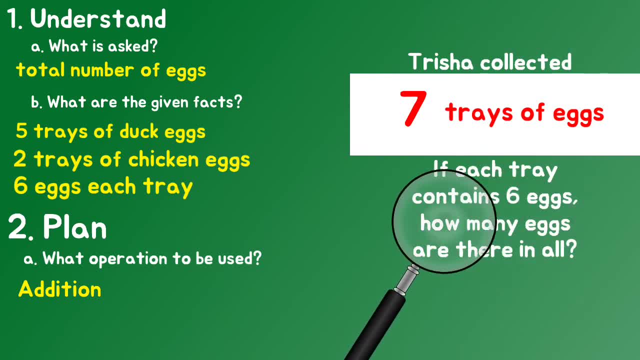 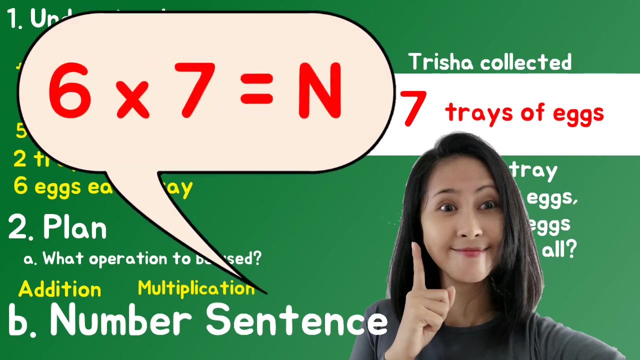 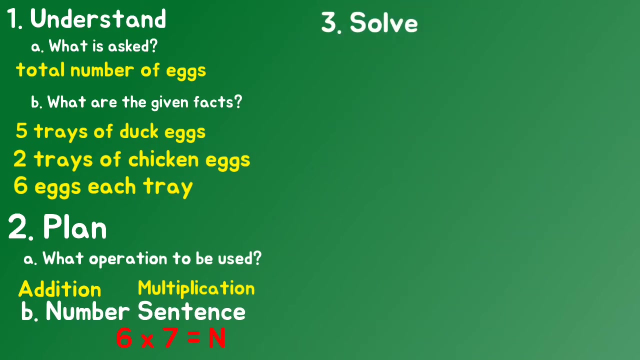 I think there are some more operational clues to the problem. Oh There, Now what does this tell us? Yes, We need to multiply. So the number sentence is 6 eggs times 7 trays of eggs. Then solve the problem. Now check, Check if your answer is correct. 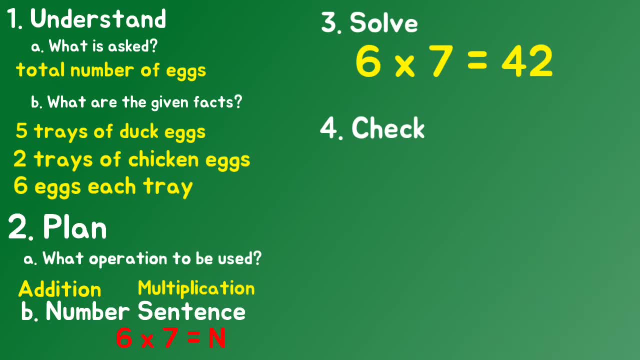 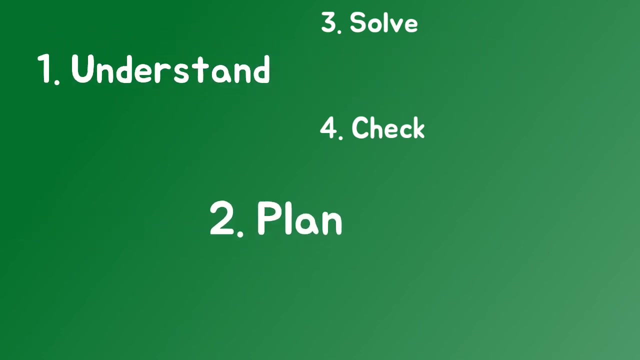 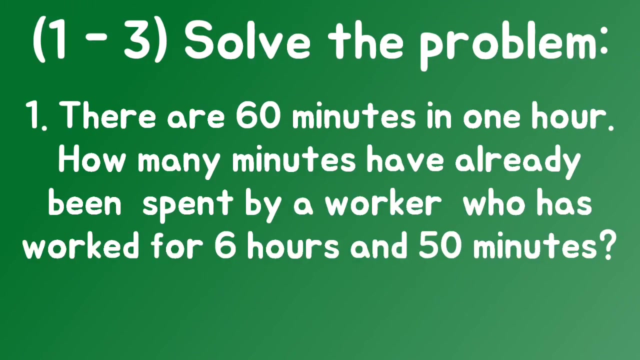 Finally state the answer: 42 eggs. What did we do to solve the problem? Understand? Yes, Are you ready? Yes, Let's go ahead. 4 eggs, 2 eggs. 1 egg- 1 egg- 2 eggs. 1 egg- 2 eggs. 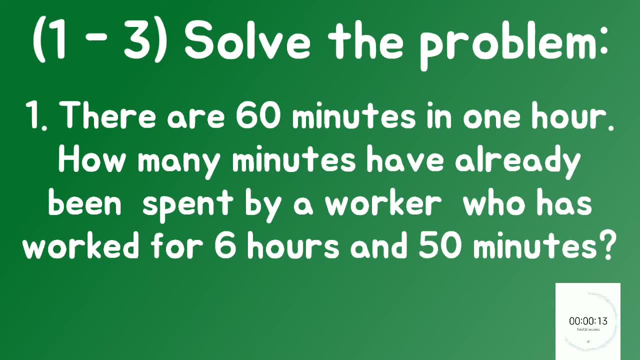 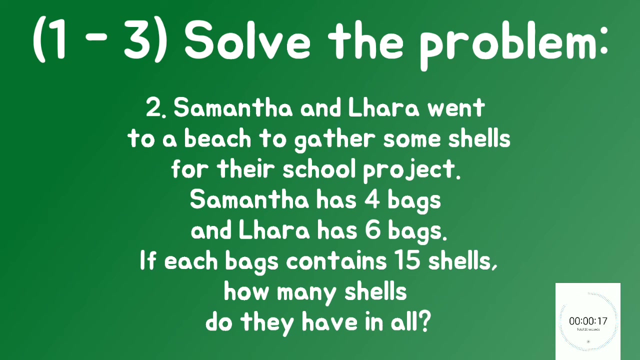 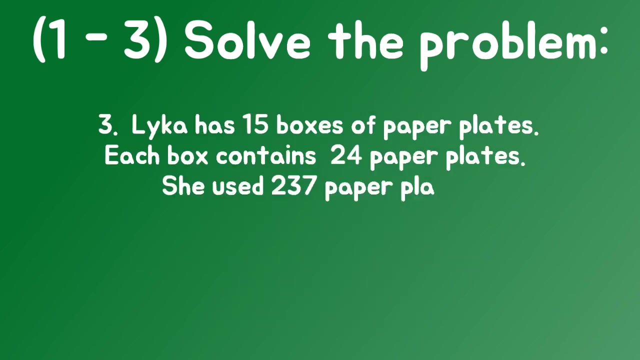 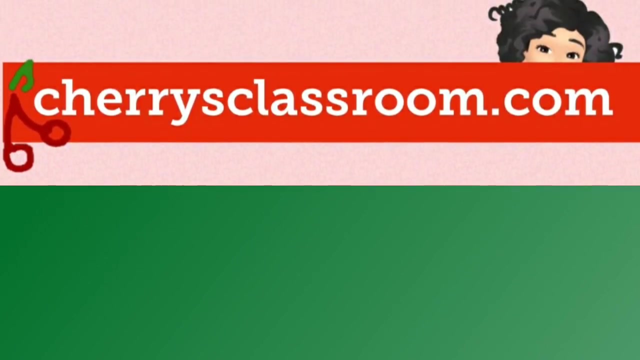 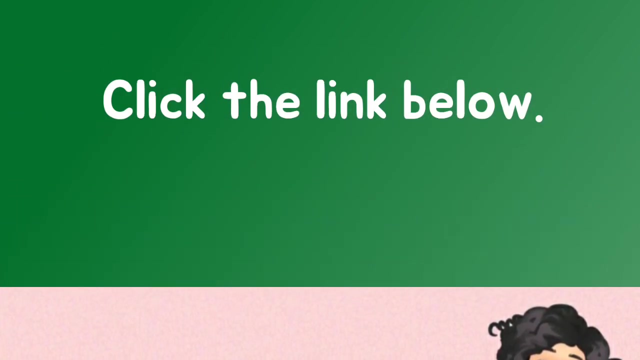 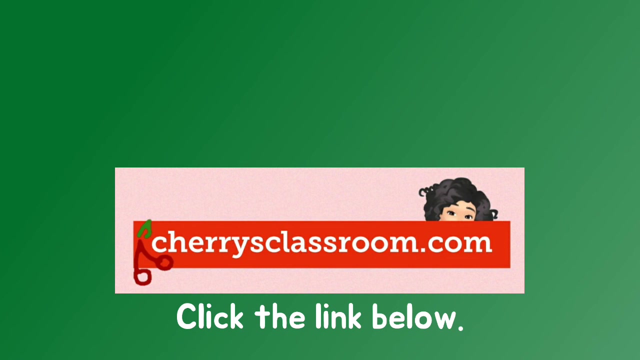